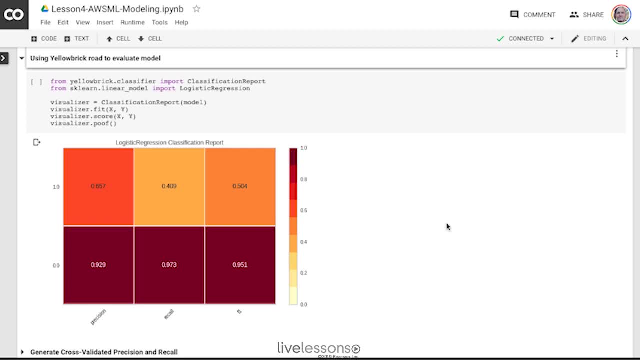 of seeing how well the model actually fits. And what we do here is we import the logistic regression and then we create a classification report. Right here we can see that this is the precision, this is the recall, and then this is the F1. And then we can actually see. 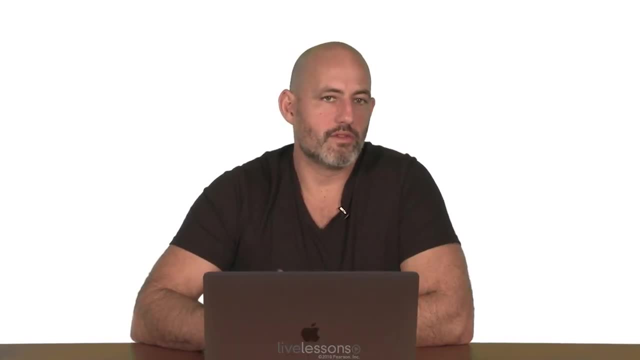 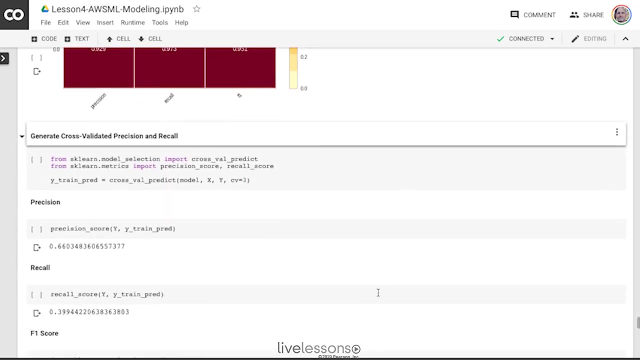 all the different reports. So again, it's very possible to be doing similar things yourself using open source software, But again, in the case of the Amazon Machine Learning Service, it does it automatically for you. Now let's go ahead and look at this cross-validated precision and recall If we wanted to explicitly 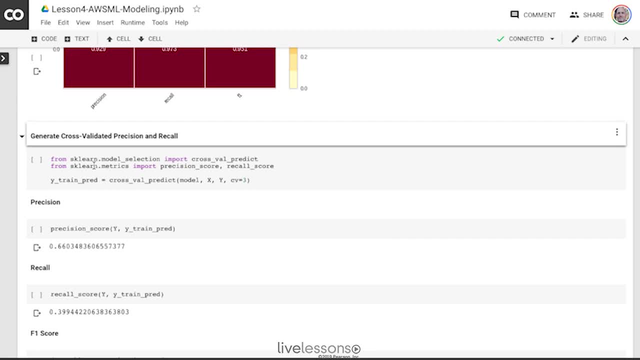 run all these commands ourself. we would go to sklearn, go to model selection, import the cross-validation, predict and then also import the precision score and the recall score. Let's go ahead and run that. There we go. Now we're able to create this, We're. 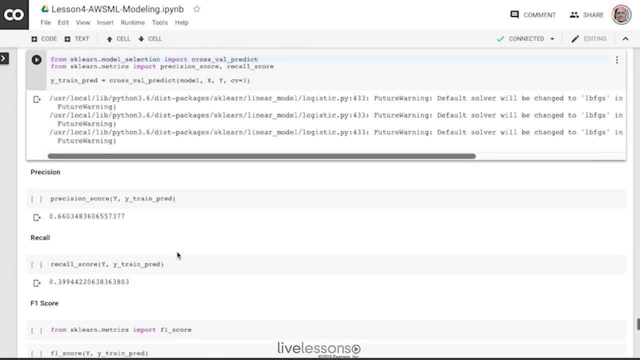 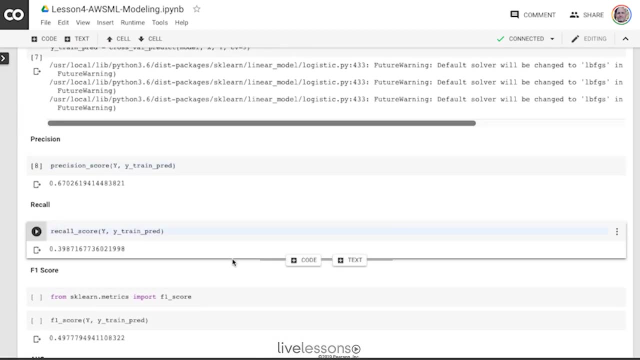 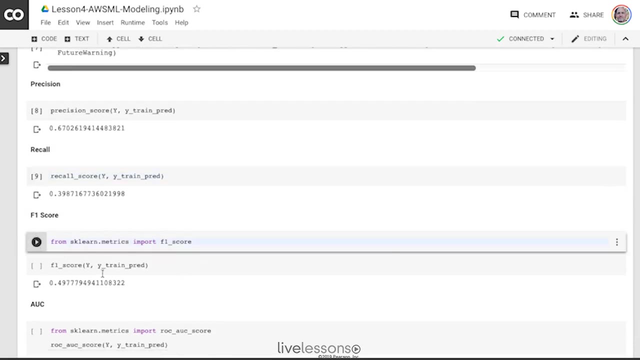 able to do Y-train prediction And now we can actually pick the precision score. Here we go. And then we can also pick the recall score. There we go. And then, if we want to go and do the F1 score, here we go. From sklearn metrics: import F1 score, We go ahead. 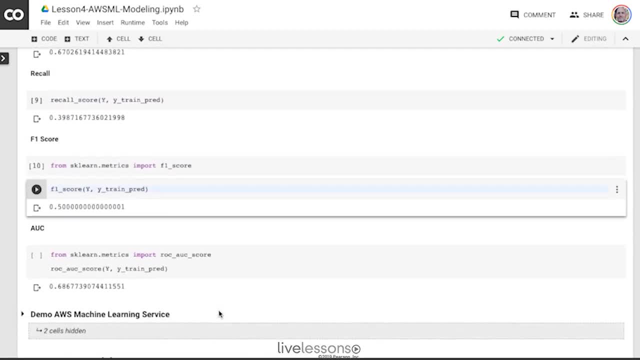 and import that F1 score And then in terms of the AUC, again the area under the curve. you can also do that with sklearn. You say, from sklearnmetrics import. And then you can also do the ROC AUC score. We pass in the Y and the Y-train predicts, And now we 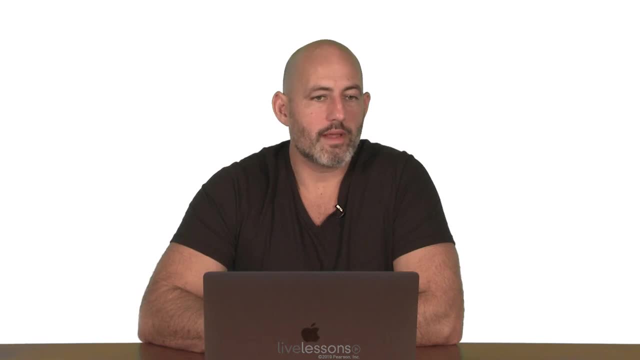 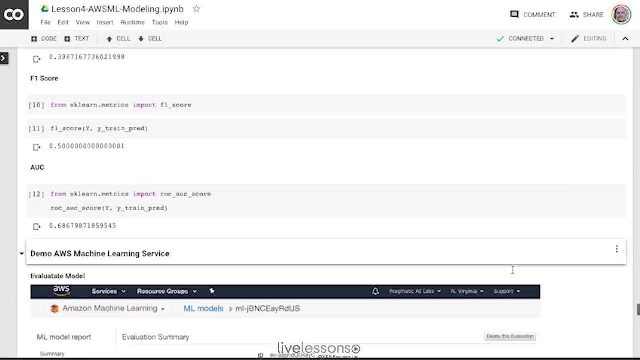 actually have the AUC as well. So great way to go through and make sure you understand things is to use this notebook and play around with all these different scores and also compare it with the Amazon Machine Learning Service. Now let's go ahead and look at what that would. 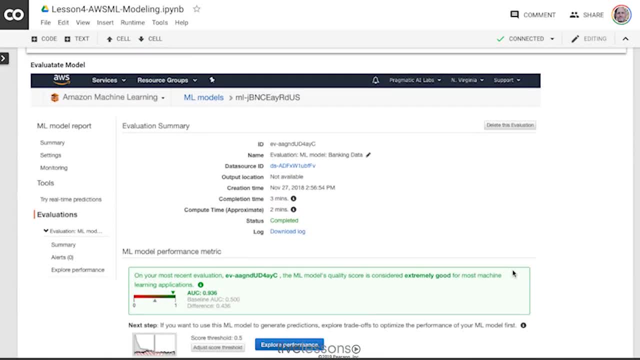 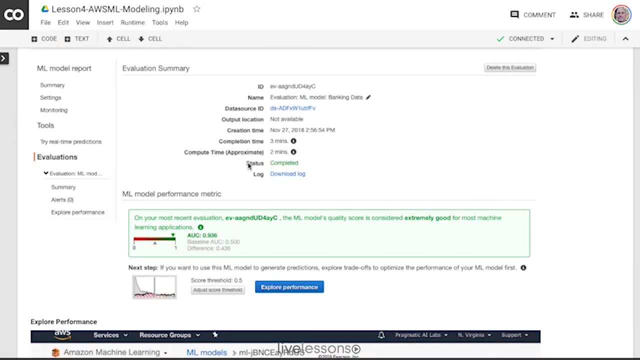 actually look like when you do the evaluation yourself. So this is the evaluation model section. And then, when you look at this evaluation model section, you'll see that there's a model performance metric here. It shows you the AUC. It also shows you again that same kind of a picture where it shows the false, negatives and false. 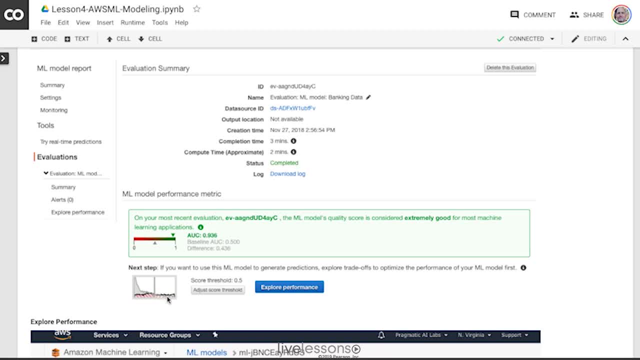 positives down here and the true positives and the true negatives on both sides, And you also have the ability to adjust the threshold yourself And you also can go ahead and explore the performance.